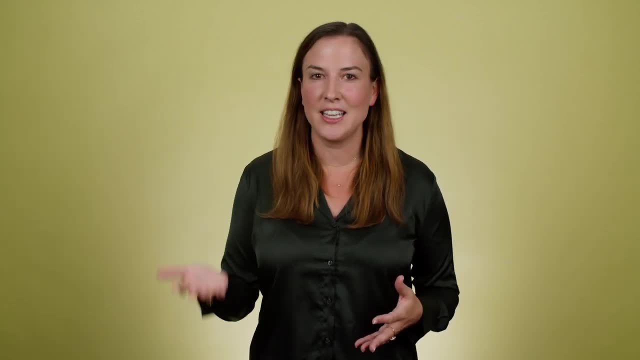 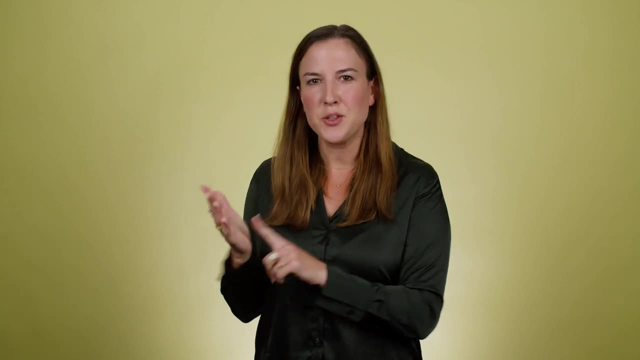 so I'm going to use this calculator. It's nice and solid, even though it's nice and light. when I pick it up, I really like the weight of it, And when I ooh, when I clack on those buttons, that sound is really. 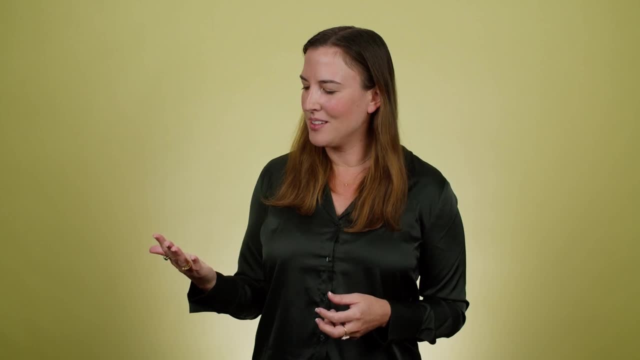 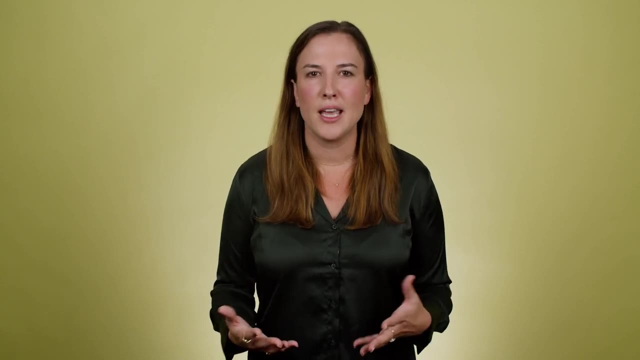 nice to hear, But the numbers on the screen are kind of difficult to read And that's going to be an issue for me because I'm often working in a setting that doesn't have a lot of light, So I think that would be a big issue for me. I like to look for a different calculator. 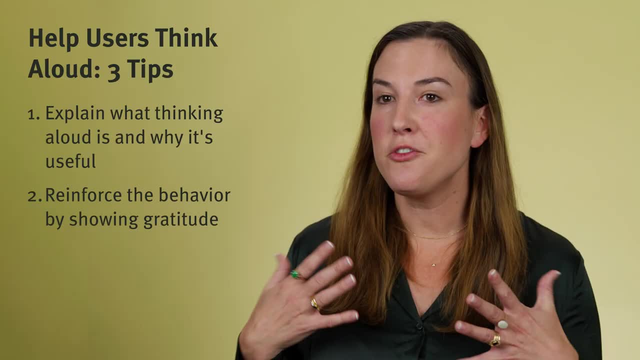 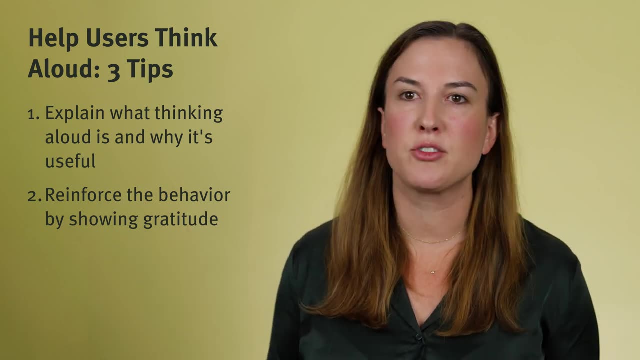 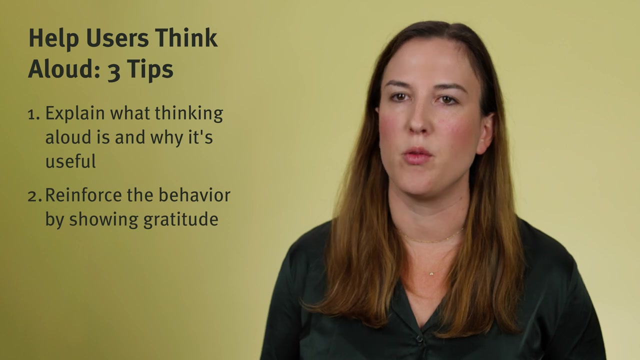 Another thing to do is just reinforce the behavior and thank participants when they give it a go At a natural pause in the test, like maybe right after the first tasks. say something like: by the way, the way you're sharing your thoughts out loud is really helpful. 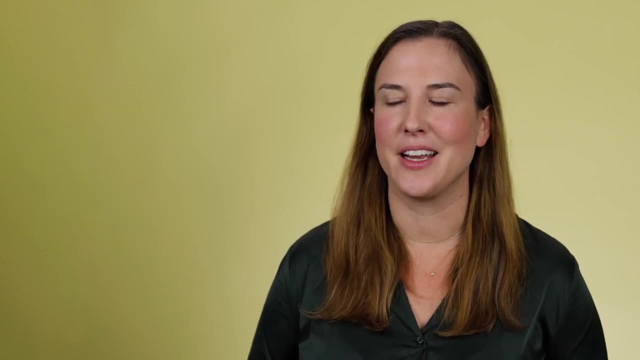 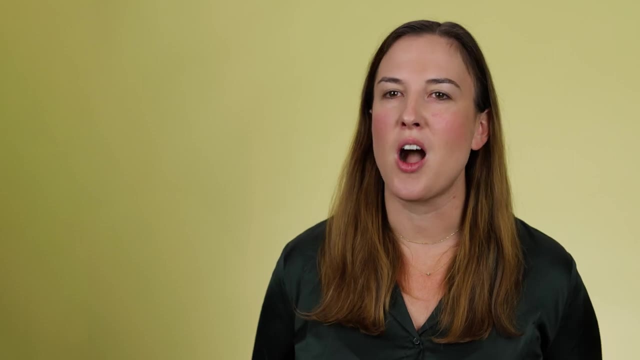 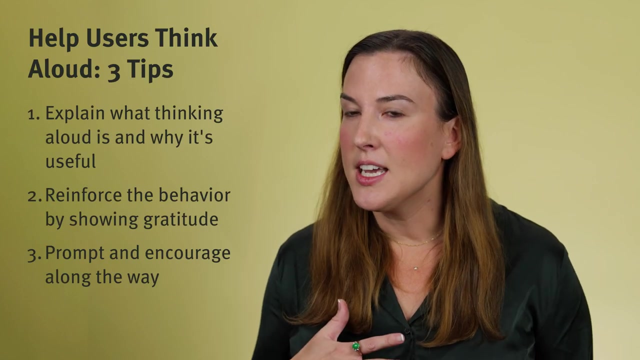 Thank you for doing that. Usually they kind of chuckle and they'll say something like: oh good, I didn't know, because it feels really weird to do that. That little simple exchange just builds their confidence. You can always prompt them a little along the way if they get quiet for too long. These 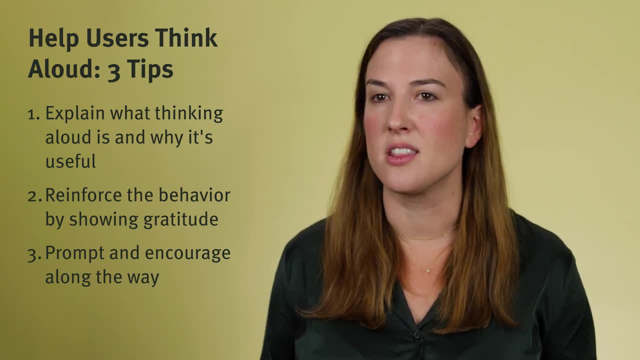 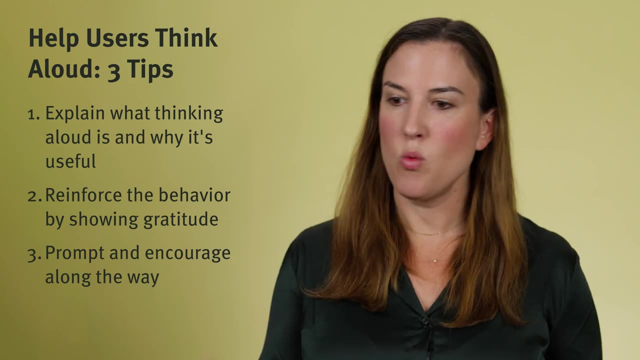 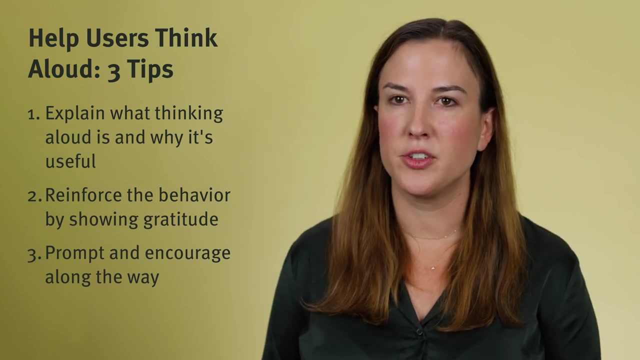 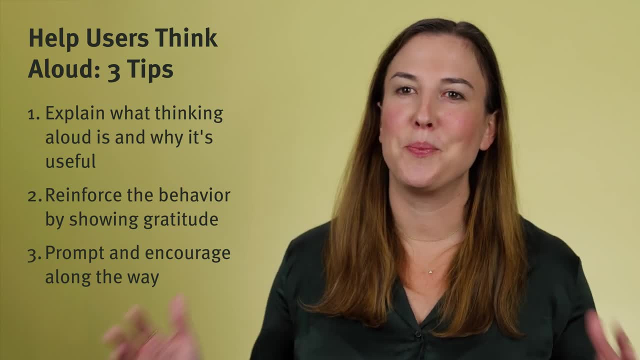 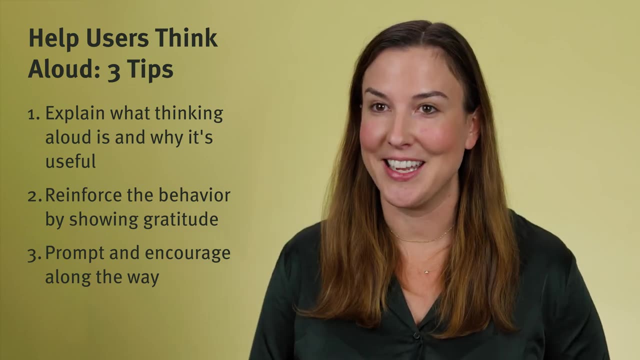 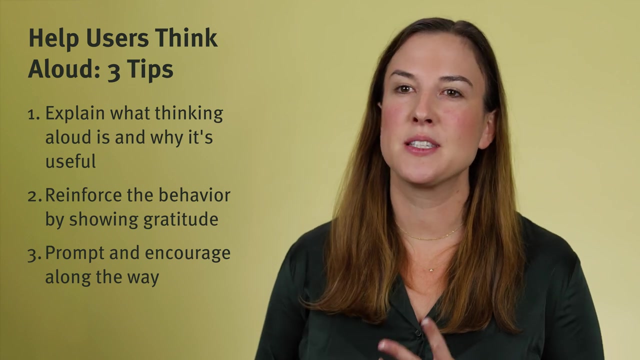 Thinking aloud is not a natural behavior. Its advantages are big. When you want to encourage participants to verbalize their thoughts, just remember to explain what thinking aloud is and why it's useful, reinforce it early and show gratitude when people do it and prompt participants to keep verbalizing along the way. 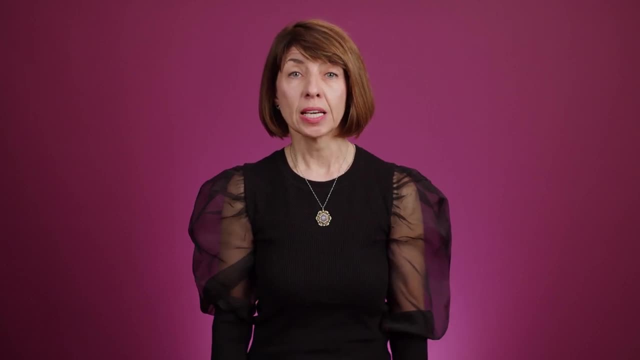 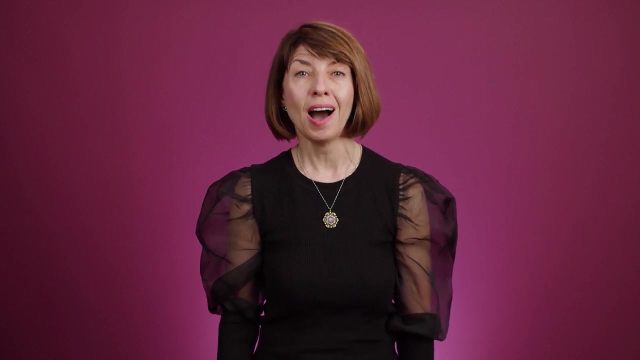 Thanks for watching. If you want to see more of our UX videos, take a look at these over here and consider subscribing to our channel. On our website, nngroupcom, you can access our free library of over 2,000 articles. 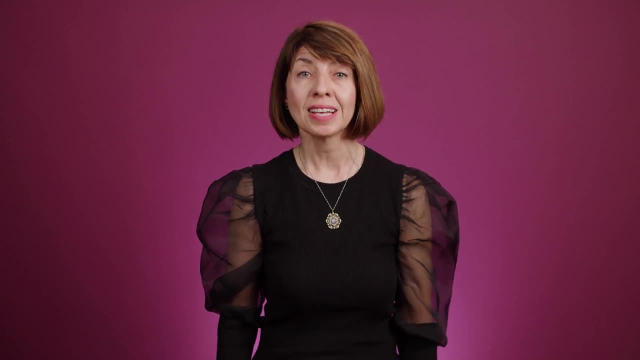 You can also register for one of our UX courses that offer live hands-on UX training.